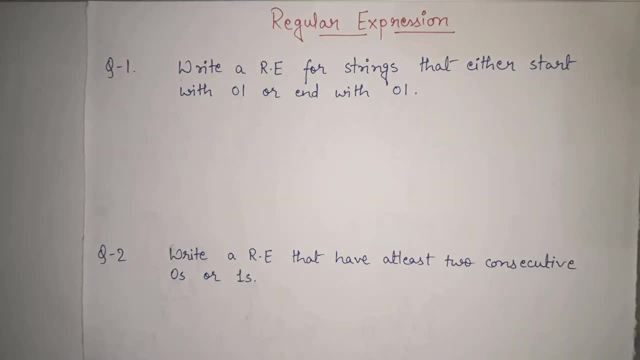 Hello guys, welcome to my channel. In this current video, what we will be seeing is what are regular expressions and how we can make the regular expression for any set of strings that is given. So first of all, here I have taken very simple example just to give you an overview that what regular expression actually are and how they can be constructed. Now, first of all, if I want to give you an overview, what is regular expression? We know that we are having 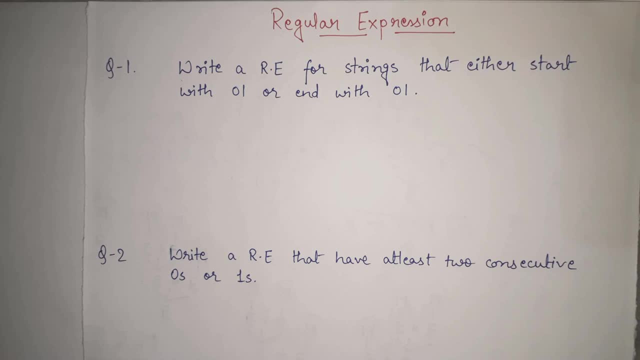 this is a topic of theory of computation, TOC right. This is a mainly topic of TOC. In TOC you must have learned that we are having main four types of grammar: type 0,, type 1, type 2 and type 3, right Now in the type 3 grammar, the type 3 grammar we are having. that is known. 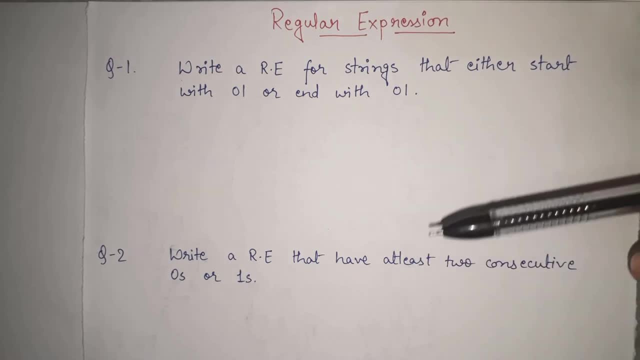 as regular grammar and the strings that are generated or the language that belongs to the regular grammar is known as regular language. Now, what regular expression is And what we know that? What is the machine to identify the regular languages? The machine we are having? 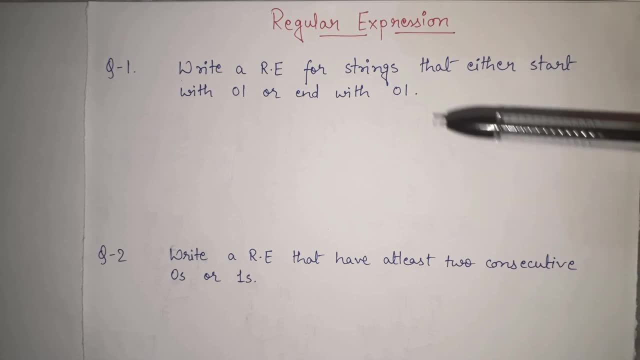 is finite automata FA. Now, any string that can be accepted by the finite automata, we can say that they are regular language or they belongs to the regular language. right Now, if we are having any type of regular language, that is, that can be accepted by any, 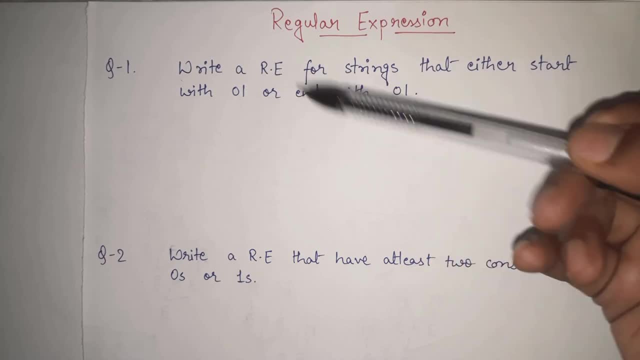 finite automata So we can generate regular expression for those particular strings. Now, what is regular expression? As the name itself indicates, regular expression it is. it will be actually an expression, a general expression that will say us that that expression it will give. 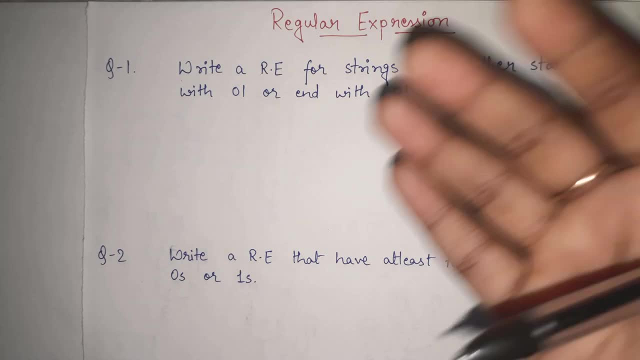 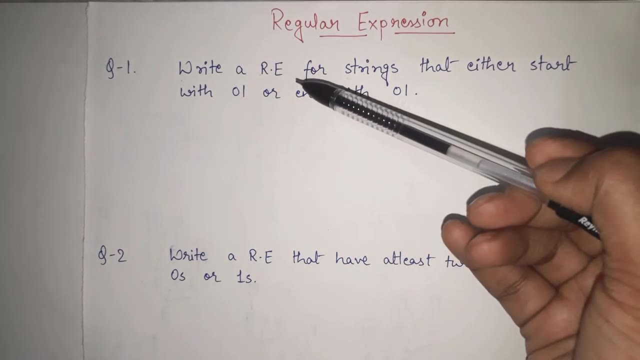 us a particular group of strings that can be accepted by that particular expression. For example, you can get an idea from the question what the question is given here that write a regular expression So clearly: 0, 1 is a regular expression, which means the string that will accept all the strings. 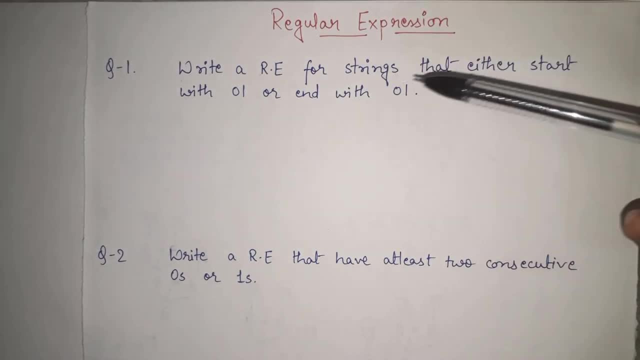 in this category must have the data of 0. 1 is the defined as the length of that string gray. We now have these two keys that we will write in the obtain sentence. We should write that at the end of the sentence, in fact that. 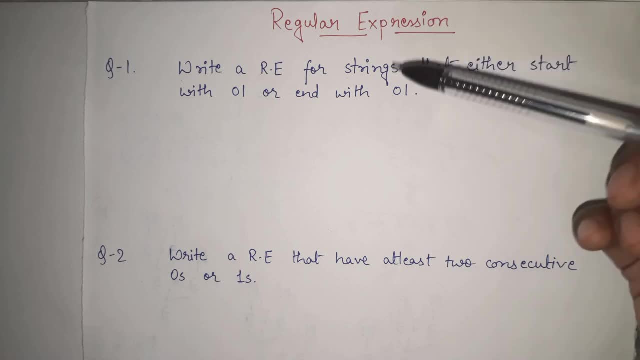 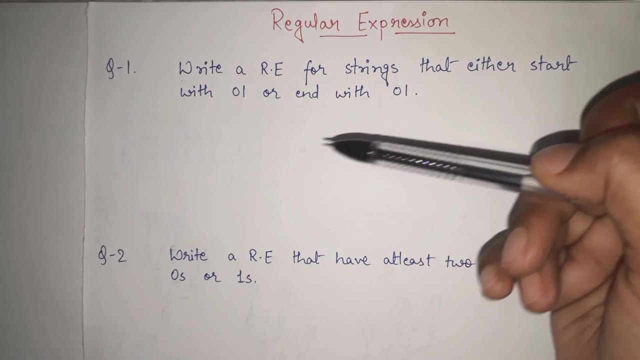 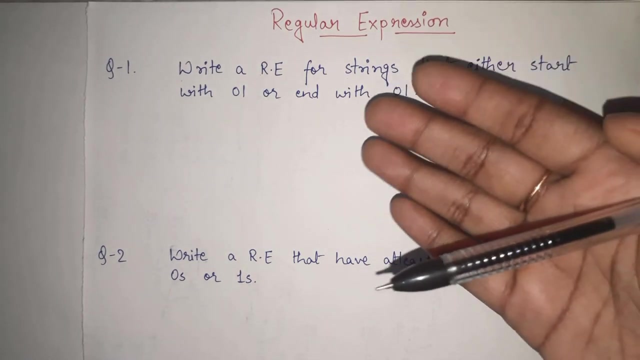 if you would clones the string by intolerance, the string will not accept it. So what forms the definite kernel of the string and what later we will write that start is equal to 0, 1.. so we are seen as second part. so we are given the state information in the terminal, but the 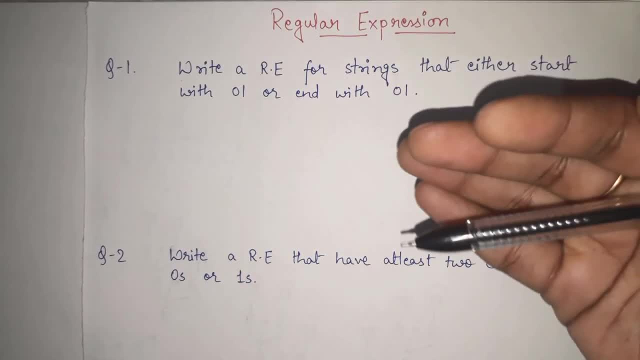 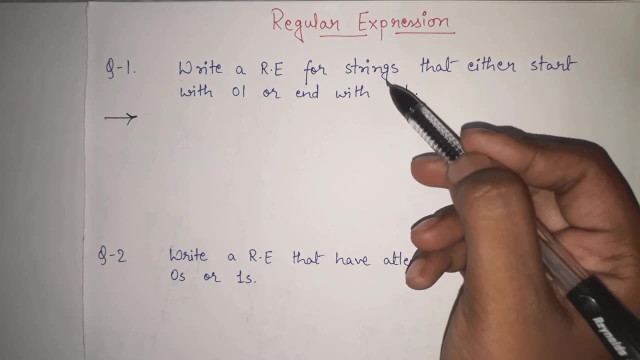 single terminal for strings that either start with 0- 1 or end with 0- 1, and this is what this is: a definition given, definition of a regular language. Now what we will be doing, idea right. So if I say about this example, what they are asking is which type of strings? 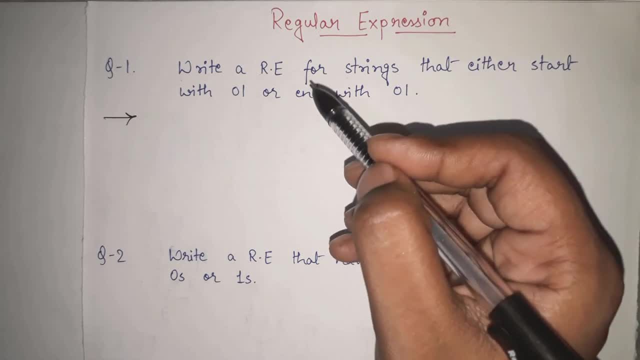 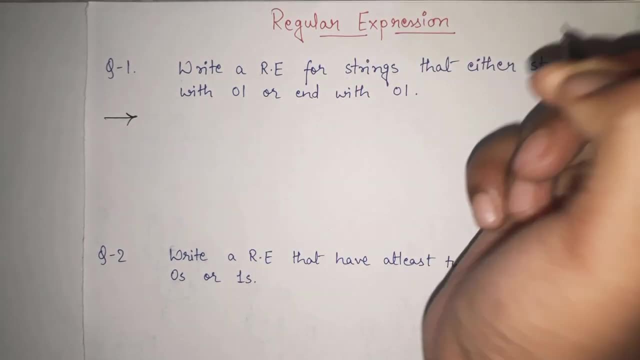 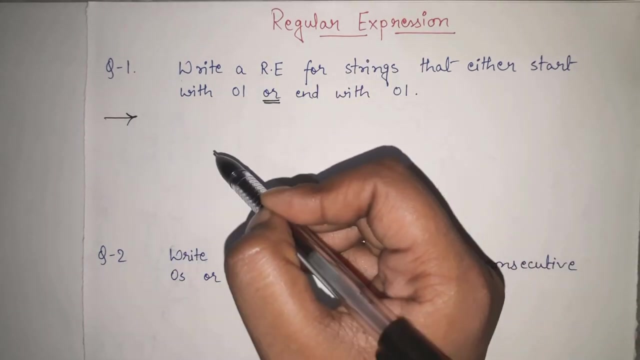 we are having. We are having the strings that either start with 0, 1 or end with 0, 1 means the see these are very small, small things that you must notice that here in between we are having- or means my string can start with 0, 1 or it cannot, or it can start with. 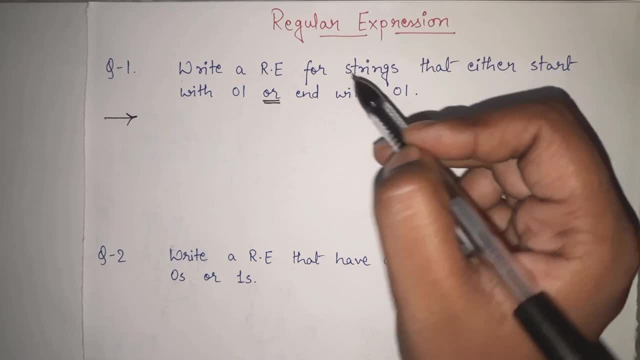 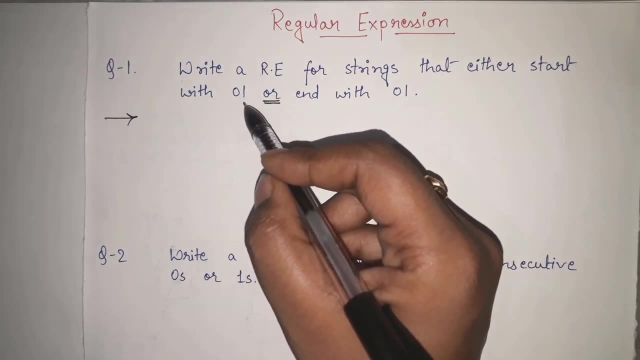 anything else, but it can end with 0, 1.. It is, or if here we would have taken and end means what. It should start with 0, 1 as well, as it should end with 0, 1, but in our case 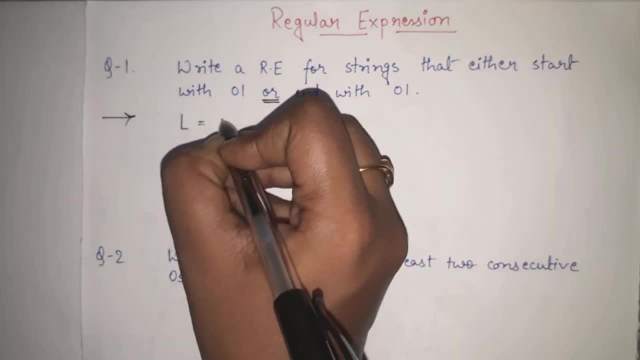 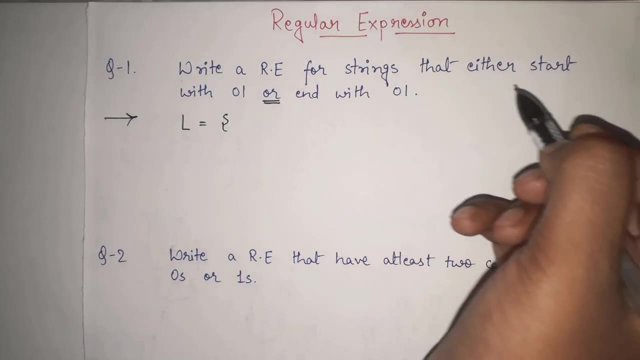 we are having, or or means: let us first write the language. that means which type of language or which type of strings will be accepted or will come in this category. again, read the question. that will either start with 0, 1 or end with 0, 1 means: 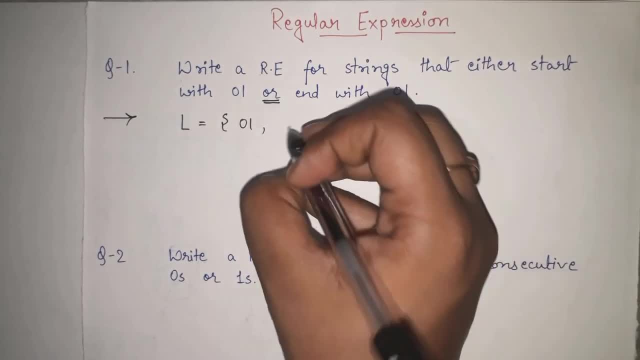 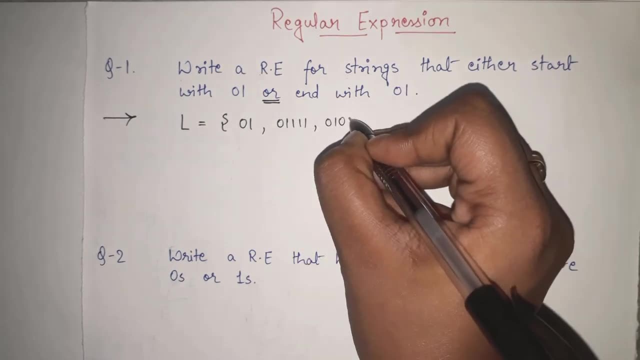 Only starting with 0, 1, it is fine. or, for example, it is starting with 0, 1, then it is having anything. it is starting with 0, 1, then it is having 0, 0, starting with 0, 1, then. 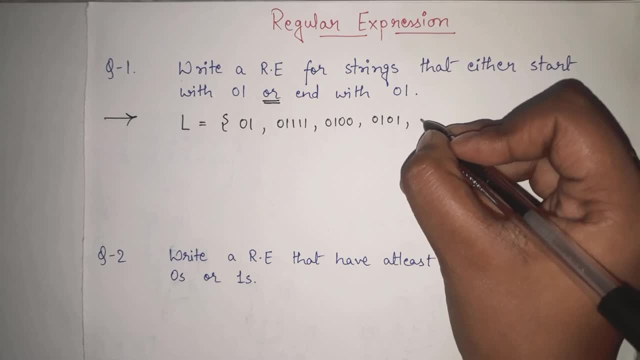 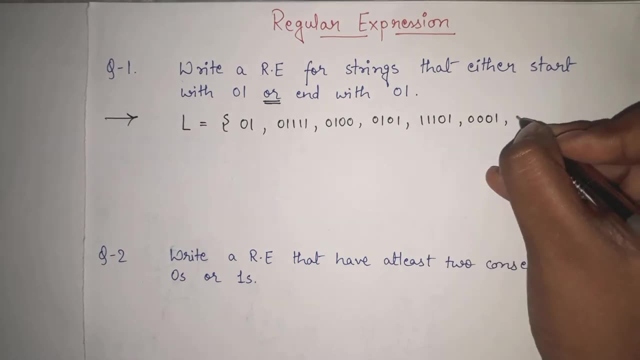 anything or end with 0, 1 means it is having anything, but it is ending with 0, 1. it can have anything but ending with 0, 1. it can have anything but end with 0, 1. fine, means what? 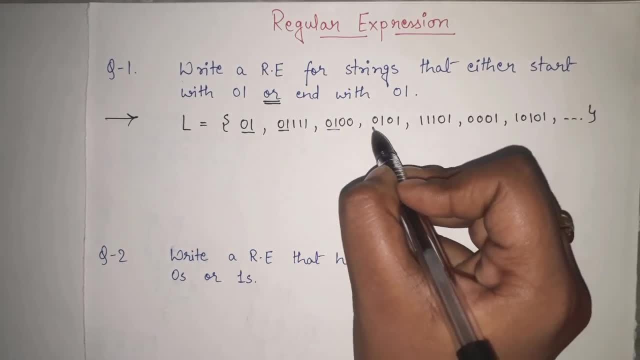 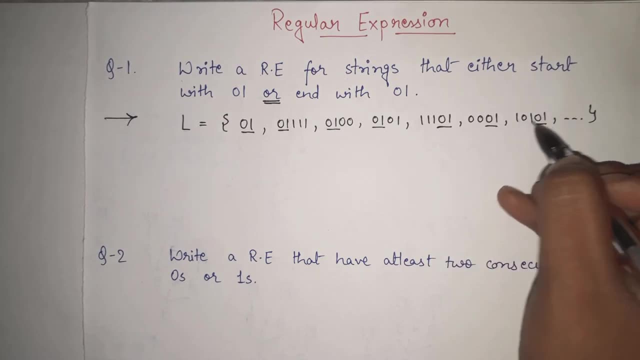 If it is starting with 0, 1, it does not matter what it is ending with, we are fine with it. or if it is ending with 0, 1, we do not care that what it is starting with, we are fine with it. but either it should start with 0, 1 or it should end with 0, 1, like this: 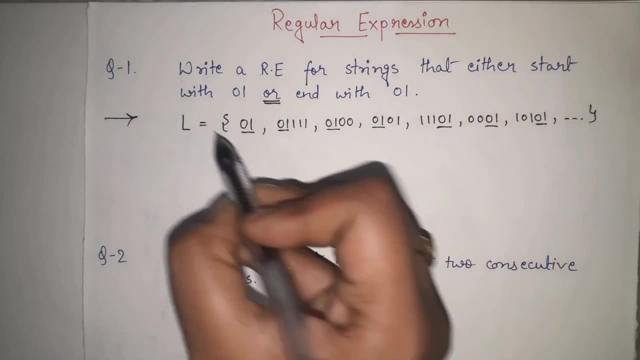 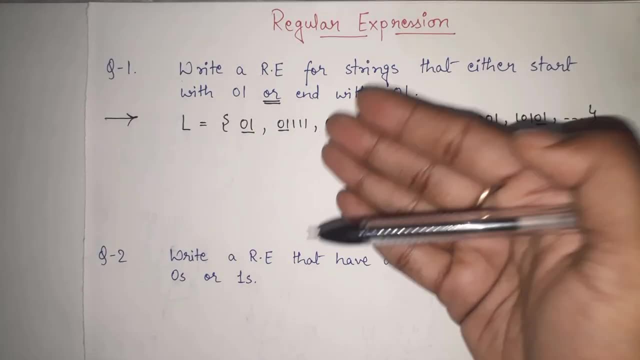 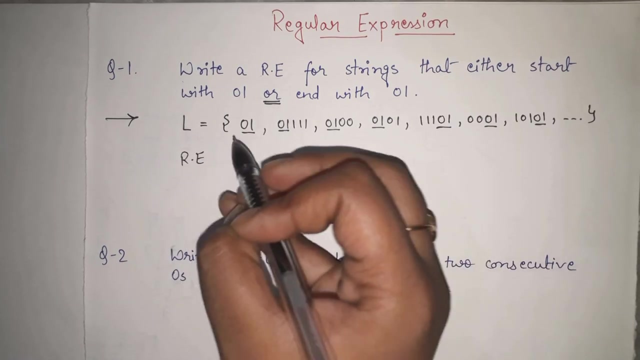 So this is our only criteria. that is given in the question. fine, so this is the set of strings or the language that I have defined. all the strings of this language are coming under this category. Now what I need to do is I need to generate a regular expression that will accept now. 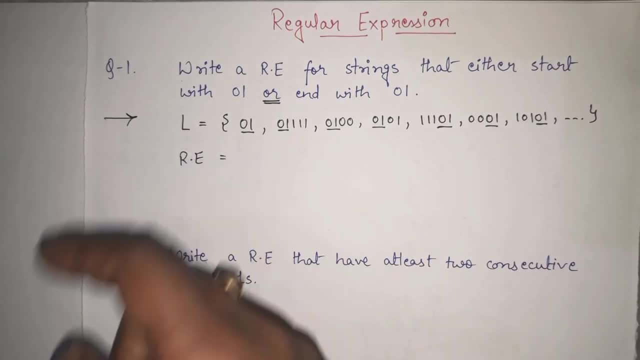 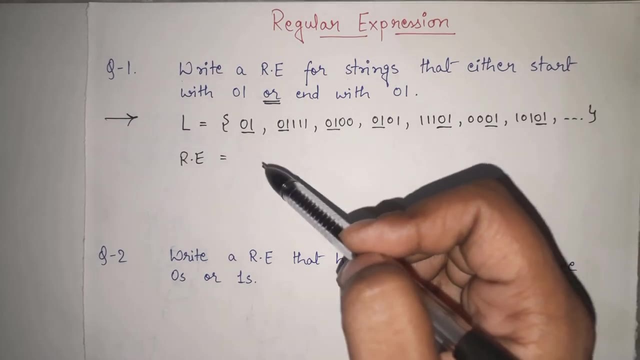 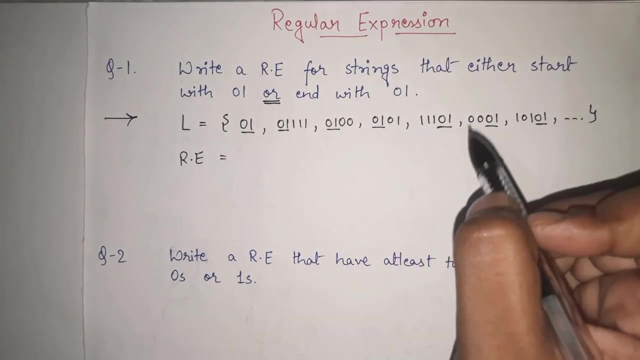 what is the main task of regular expression, or what is the main characteristic that this regular expression that I will be generating here? it should accept each and every string that belong to this language, and it should not accept anything, any such string. it should not accept any such string that does not belong to this L. 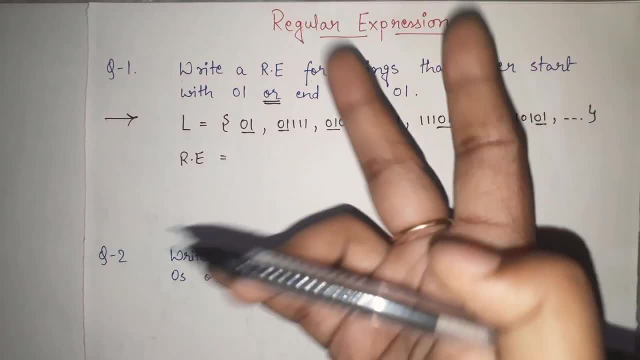 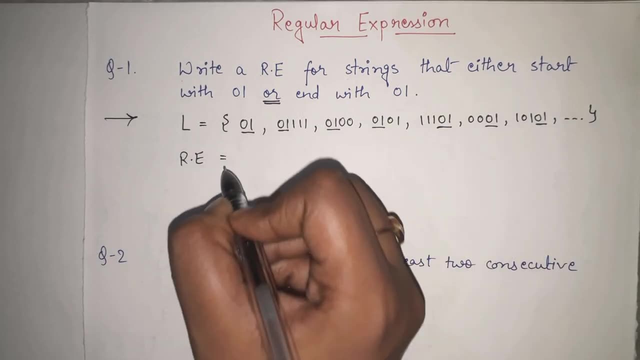 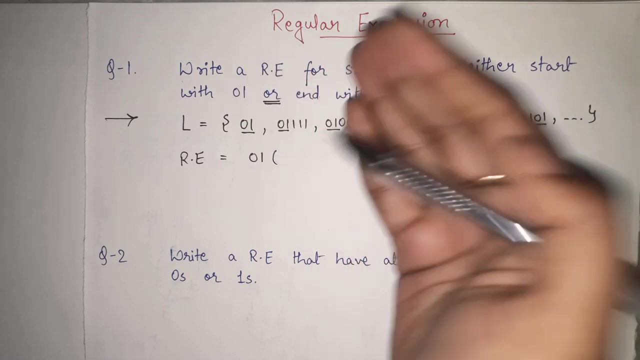 That does not belong to these set of strings, right? so we have to check both the cases. Now, if I start making the regular expression for this language what it is saying, it will always start with 0, 1. it is starting with 0, 1 then, whatever is there behind it, it does. 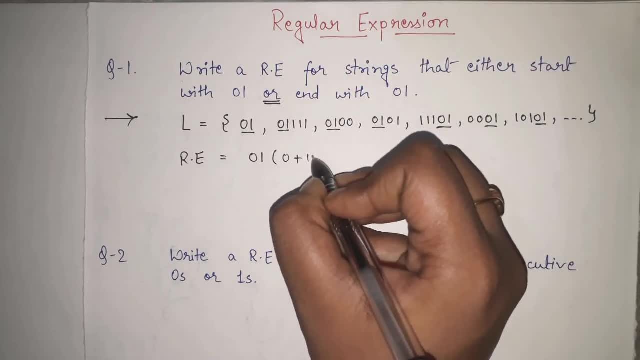 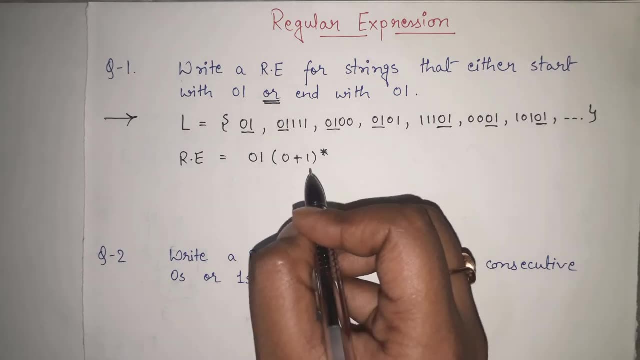 not matter. so 0 or 1 star, what is 0 or 1 star means? it means any combination of 0 and 1, means if it is starting with 0, 1, then after 0, 1 any combination of 0, 1 is there it does. 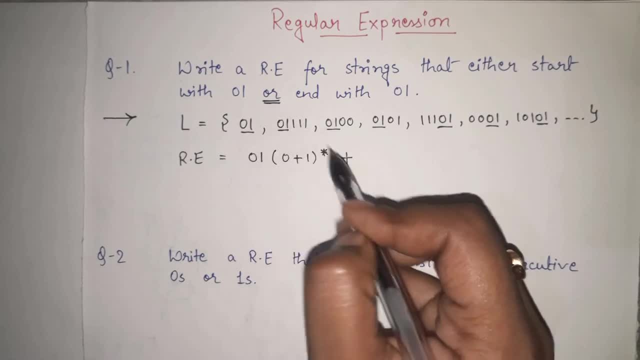 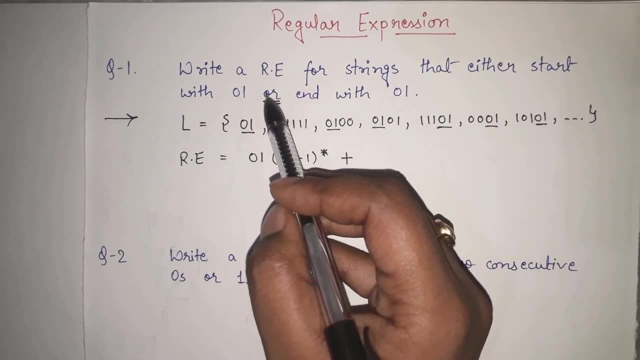 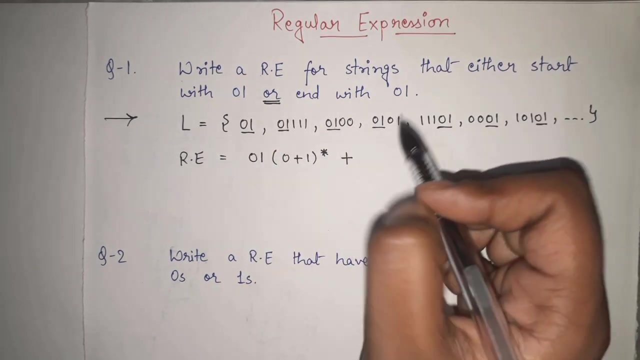 not matter, or whenever we are having, or in between. or is indicated by plus sign if it is. if it was, and then what we would have written dot? dot represents and, but in our case it is, or. so we will be writing plus, or, and with 0,. 1 means if the string is ending with 0,. 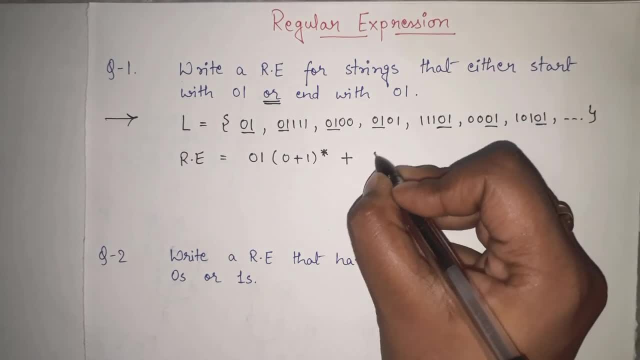 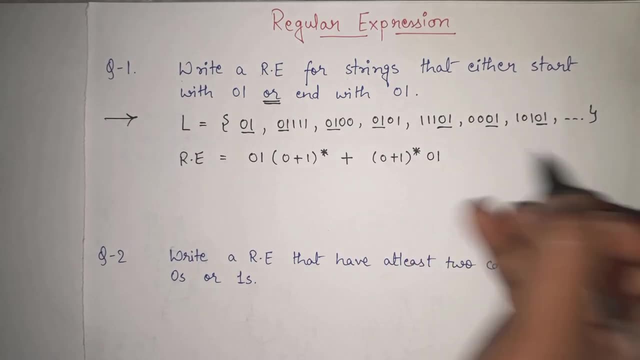 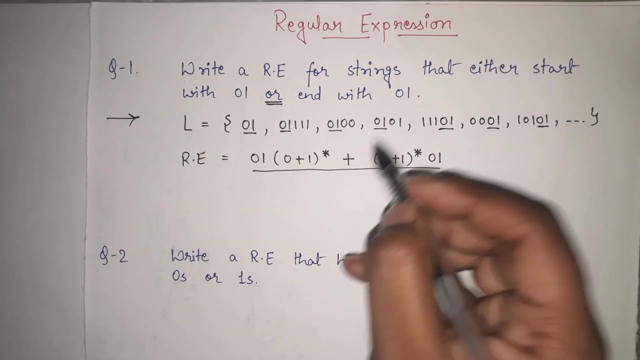 1. So what is there in the beginning? it does not matter. so in the beginning we can have any combination of 0s and 1s, but it should end with 0, 1, so either this or this. so this is my overall regular expression that accepts all the string that either end with 0, 1 or 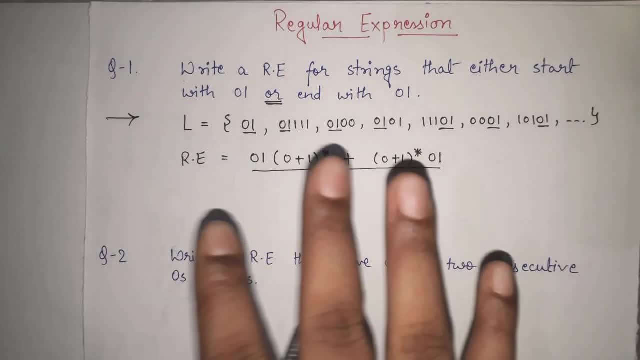 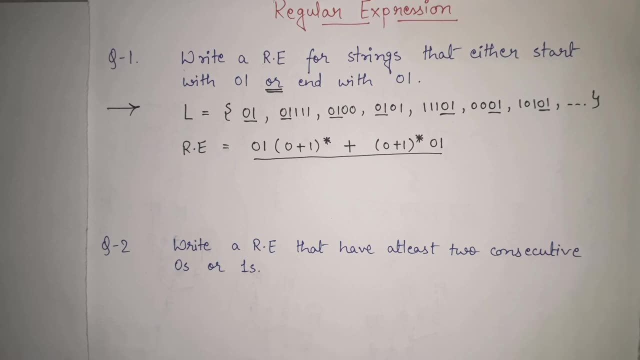 start with 0, 1. fine, I hope you have understood. it is actually very easy. Okay, now coming to the second question. we have to do the same thing here. here the question is: write a regular expression that have at least two consecutive 0s or 1s. what do you? 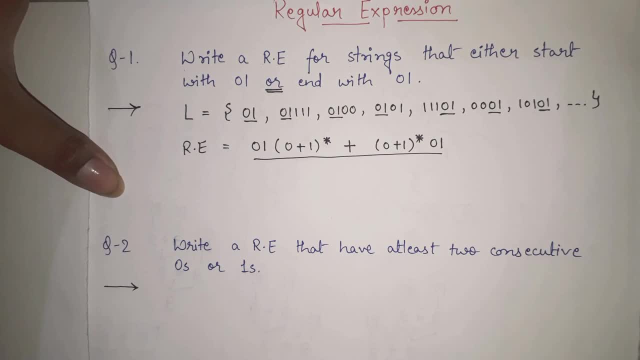 mean by consecutive 0s means two 0s will be together or two 1s will be together, at least two consecutive 0s or 1s together. so my language will contain the strings like 00 or 11, because at least two must be there, at least two, or we can have three consecutive, four consecutive. 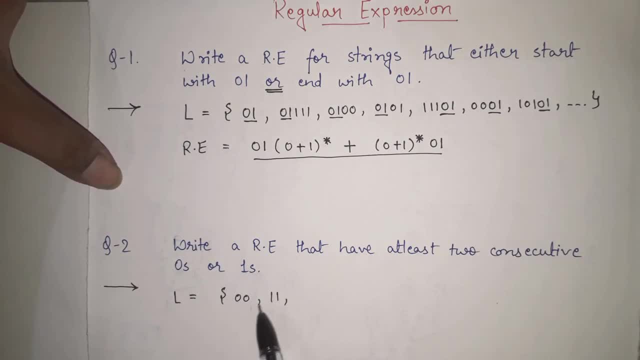 five consecutive, it's fine, But at least two consecutive 0s or two consecutive 1s, Okay. Or two consecutive 1s should be there here also. we are having all fine. so we can have 00, then any combination. we can have 11, then any combination, or in between also we can. 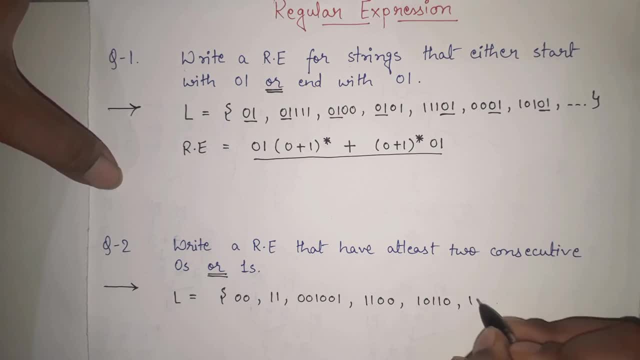 have two 1s right. or, for example, I am having all 1s but two 0s here. I am having 1010 here, two 0s, then 1, any such strings I can have, that can, that is, containing either consecutive 0s or consecutive 1s. 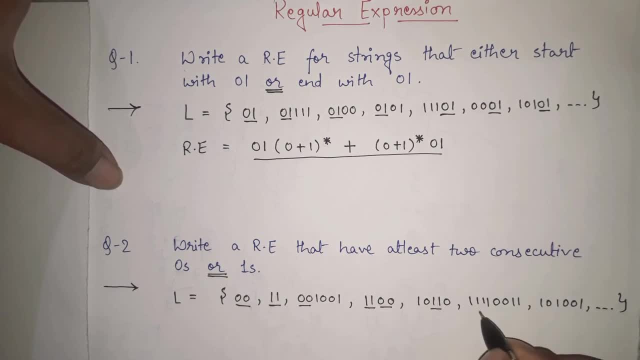 0s, 1s here, 0 is also there. 1, 1s, 0s, 0s. any combination of either 0 or 1 is fine with our string, fine. So these are again the set of strings that can be accepted by this. 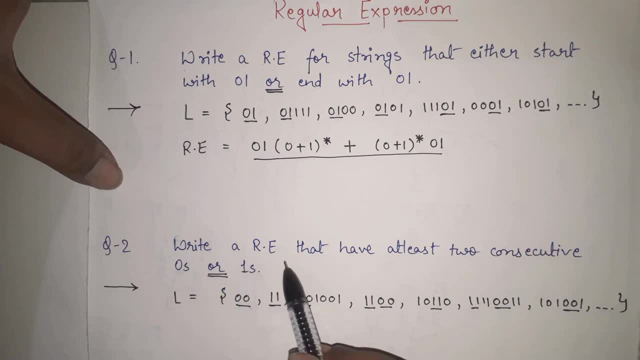 given definition that is given to us, that regular expression for the strings that will have at least two consecutive 0s or two consecutive 1s. Now regular expression for this, how we will make it Here. also, one thing is clear: that in between we are having or so in between, 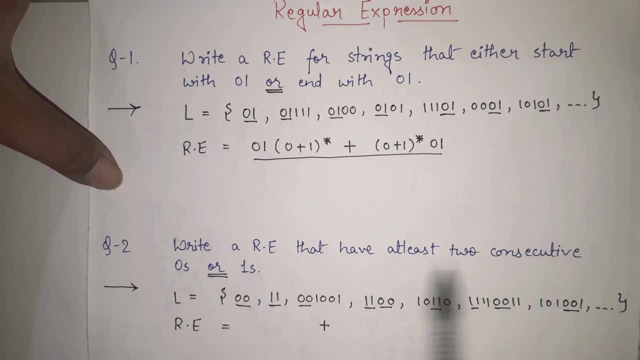 we will be having plus sign. Now, two consecutive 0s or two consecutive 1s means what? Any combination of 0s and 1s, but then two 0 and again any combination of 0s and 1s. let me write it. 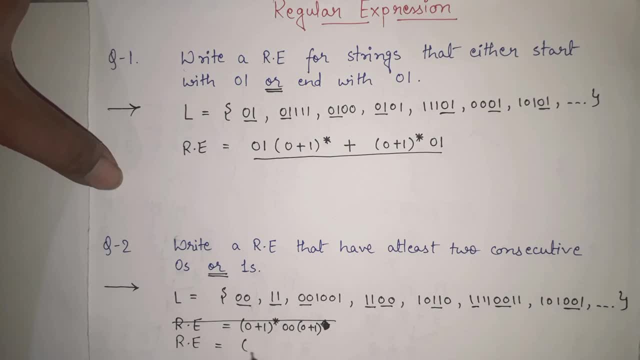 again here, that any combination of 0s, that any combination of 0s and 1s, then two 0s, then any combination of 0s and 1s- fine, So this will give me at least two. 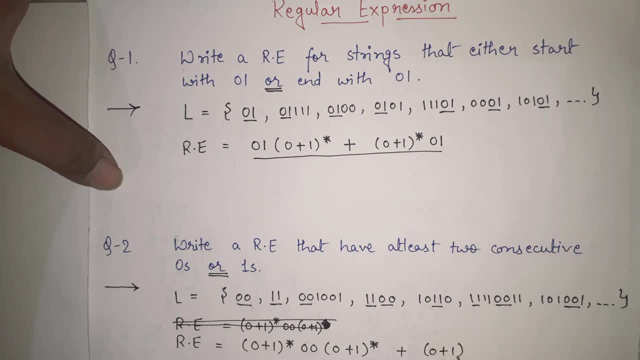 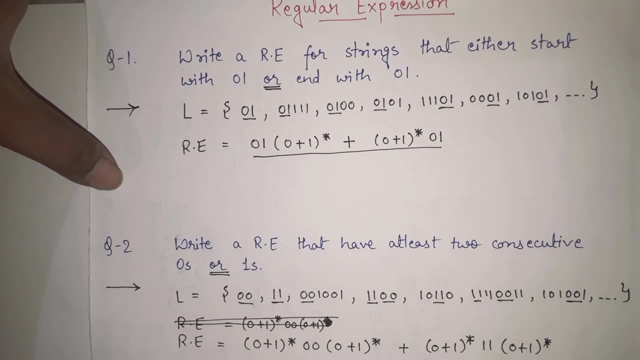 consecutive 0s, or any combination of 0 and 1,, two 1s, then again any combination of 0s and 1s. So it will give me what? At least? two consecutive 1, and it will give me at least.